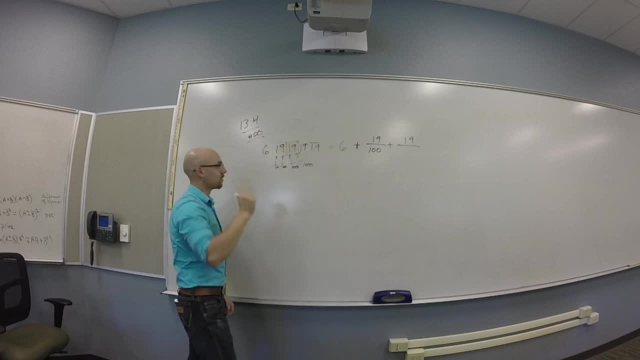 And I'm just talking about this guy here- right, You wrote 1,000.. Sorry, I can't keep track of zeros. So that's 19 in the ten-thousandths place, right? And how does 19,, or how does 10,000, relate to a hundred? 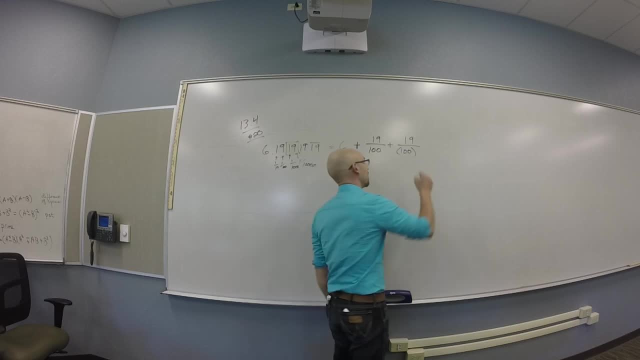 I don't know, Relate to a hundred. It's a hundred squared, It's a hundred squared. And then the next one is going to be 19 over. and what's this place here? That's the A hundred cubed. 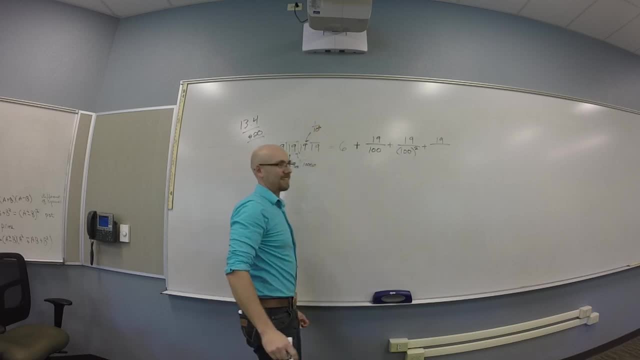 Yeah, that's 1 over 10- to the sixth right, which is a hundred cubed and so forth right, And so then I think you should split it right. I think you should split this into two pieces. So I'm going to split this into the sixth right. 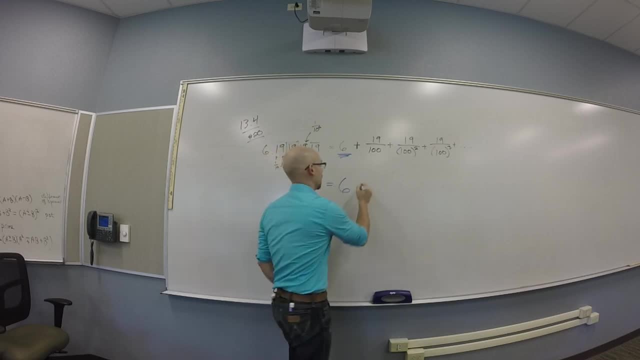 So there's a sixth, and then I'm going to: oh, I need to write that thing as a geometric right, Okay. So what have I got there? There's a 19, right, Mm-hmm, There's 19,. and then I'm multiplying 19 by 1, over 100,. 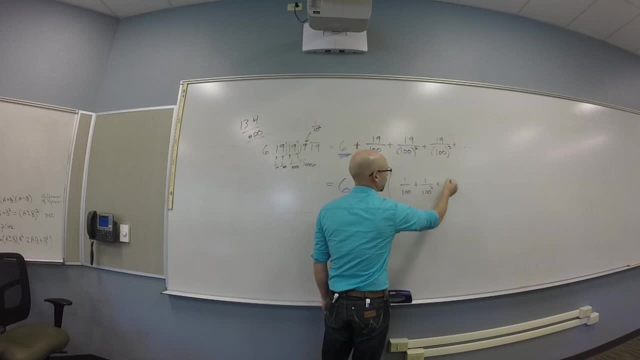 plus 1 over 100 squared, plus 1 over 100 cubed, and so on. right, So it would be 19 parentheses, 1 over 100 to the power of 10?? Yeah, So this whole guy. right is the sum. 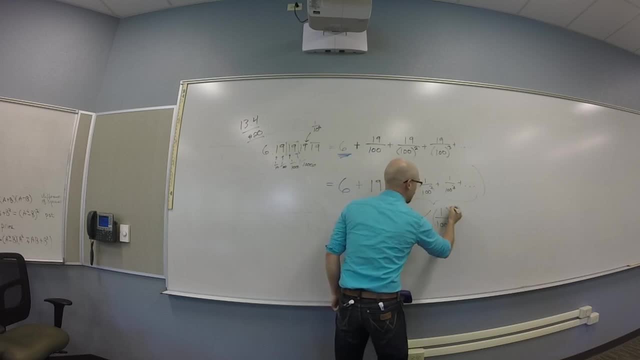 of 1 over 100, all to the power of n, and I'm starting at n. is what? So just that piece? what power of 100? am I starting? 1 over 100? am I starting 1. 1?? So we're going from n is 1 to infinity. all right. 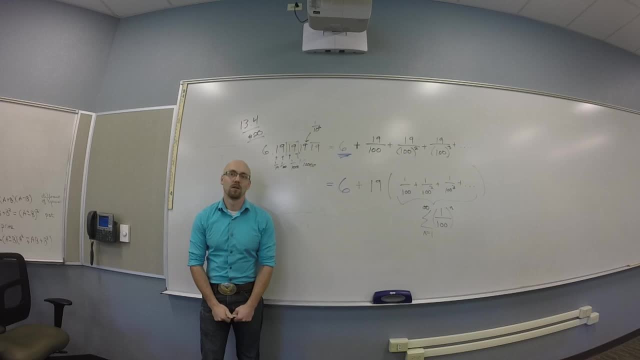 You guys with me, You could also write it as 100 to the power of negative n Totally. I would recommend it this way, because this way is the one I have the formula for. Or you can just make a new formula. You guys remember where the formula starts yet. 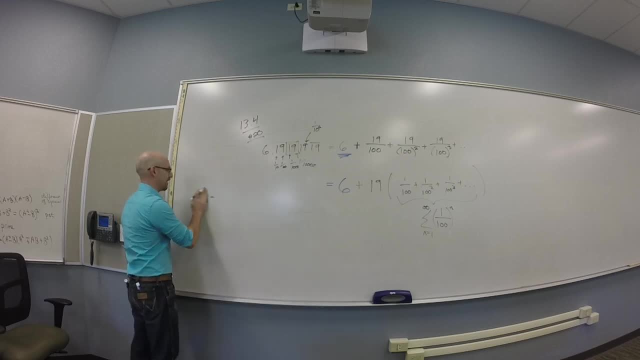 So I have this thing right that I developed the other day, that there's a sum of r to the n's from n is something to infinity, and that gives me 1 over 1 over 100, right, Yeah, Yeah. 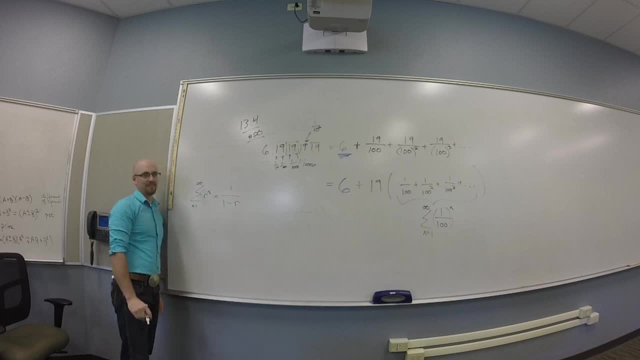 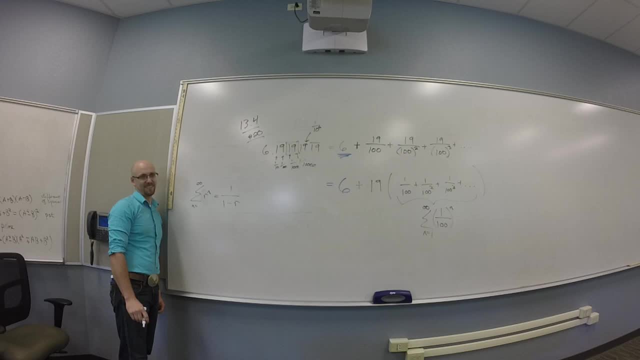 You guys remember this one: Where does this one start? Starts at zero. Yeah, good, This one starts at zero. Does that thing start at zero? No, No, no. That one starts at one right, Because if it started at zero, then 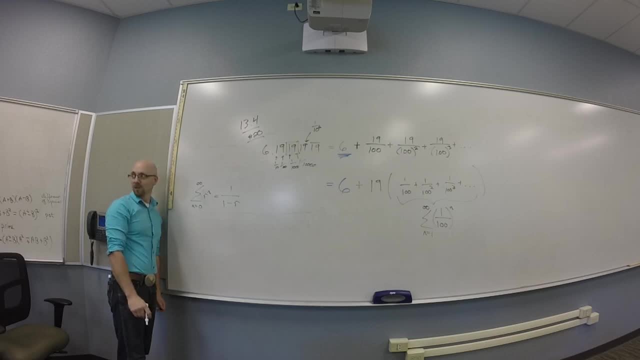 If it starts at zero, then I could just use this formula. You guys got that, Yes, maybe Okay. so how do I make it start at zero? What do I need to do? Minus 1.. Yeah, I need to take this thing right. 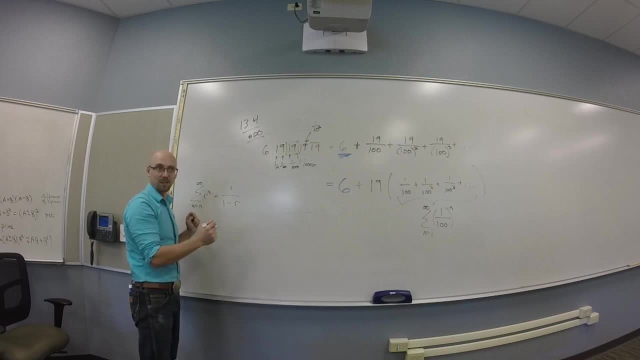 subtract the first term off of it. See that. So if I subtract 1 from both sides here, right, then I'll have the sum from n is 1 to infinity, of r to the n, and that'll be this: 1 over 1 minus r and then minus 1.. 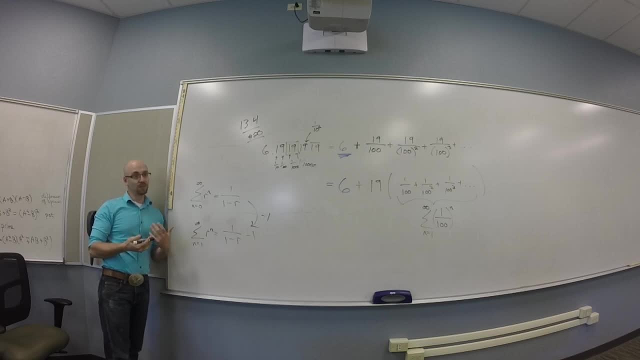 You guys see how I modified this thing. If there were several missing, right, I'd just subtract all the ones that were missing. So if there were 2 or 3, then I'd subtract 2 or 3.. A better idea might actually be to factor out of this. 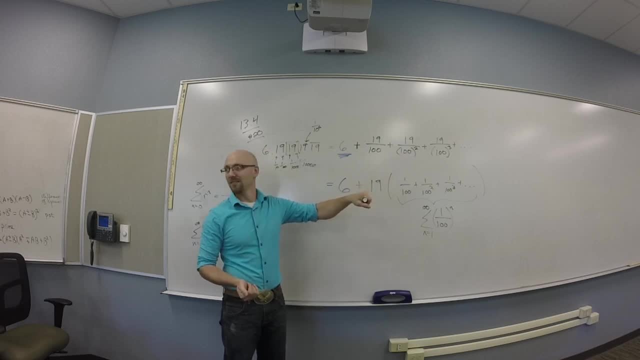 I could factor out 1 over 100. So if we have 1 over 100.. So if I factor out a here, I factored out a 19,. right, because there was a 19 in the top of everything. Well, there was a 100 in the bottom of everything too. 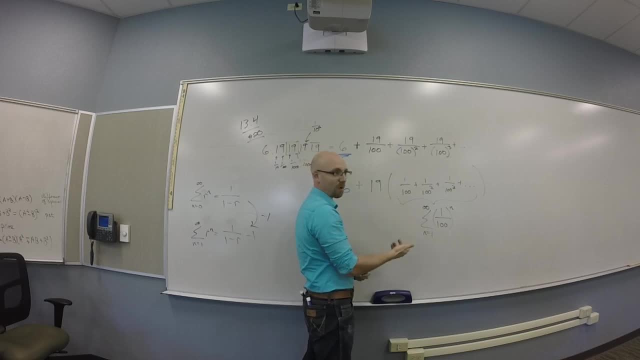 So I could have factored out a 19 over 100, and then I wouldn't be dealing with this problem. So maybe not 19 over 100. Yeah, whatever. So I would just go ahead and use this, since we developed it.